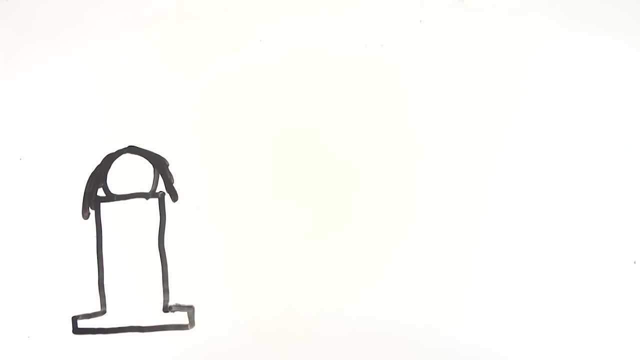 essentially a survival of the fittest society. On the political spectrum, the Democrats and Republicans tend to have opposing positions on matters such as the economy, society, military and other key issues. Both political parties are so large now that it is quite hard to work out where their positions are on certain 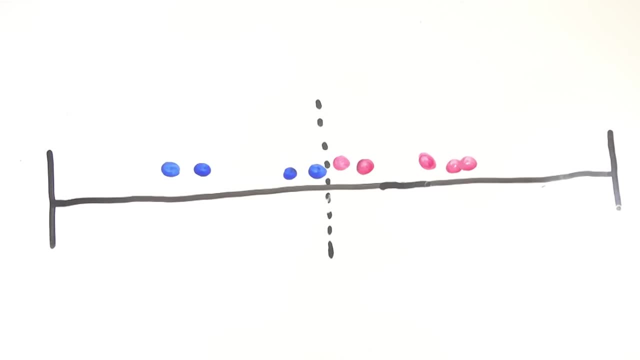 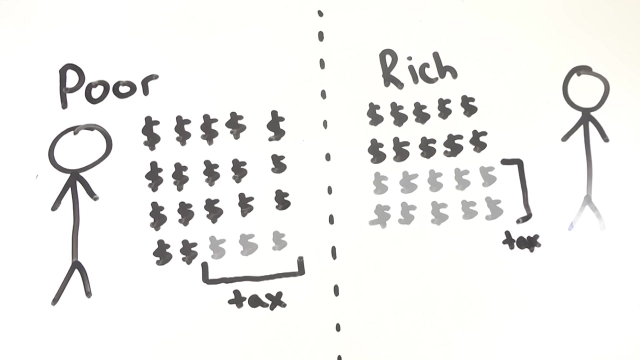 issues, but there are a few key issues where their opinions are quite apparent. but even then, candidates within the same political party can have slightly differing views on major issues which affect us all: Taxation. When it comes to taxation and wages, the Republican party believe that high taxes on the rich is a form of class warfare and that both the 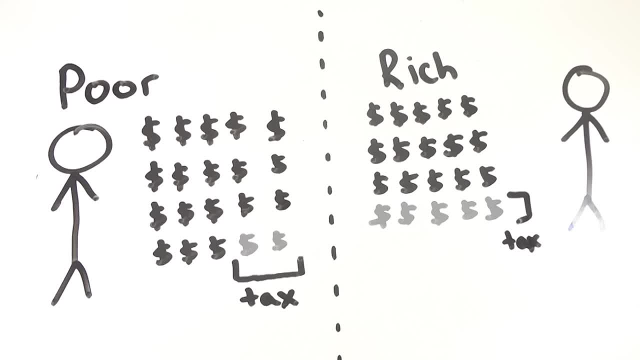 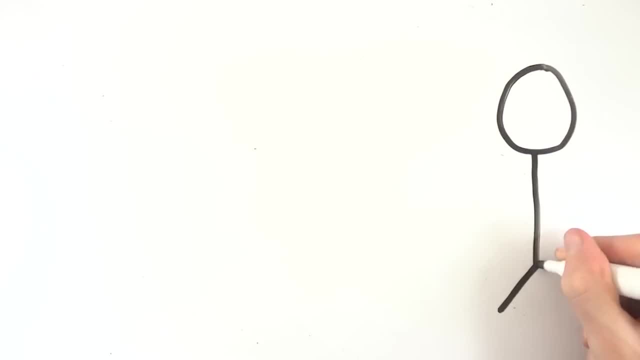 poor and the rich should receive tax cuts, As the Republican party's plans would see the revenue which the federal government collects decrease. the results would be higher debt and deficits. By lowering the taxes for the upper class, these people are more likely to invest in businesses, which in turn creates jobs, making a trickle down effect. Republicans. also oppose raising the minimum wage, as it believes it hurts small businesses, who account for a large amount of employment for Americans, Taxes on the rich are a form of class warfare and that both the poor and the rich should receive tax cuts, As the Republican party's plans would see the revenue which the federal government collects decrease. the results would be higher debt and deficits. Democrats, on the other hand, believe in raising taxes for the upper class and lowering taxes for the middle and lower classes of society, allowing the government to boost their spending on social programs for the lower class. Simply put Republicans: lower tax to benefit the 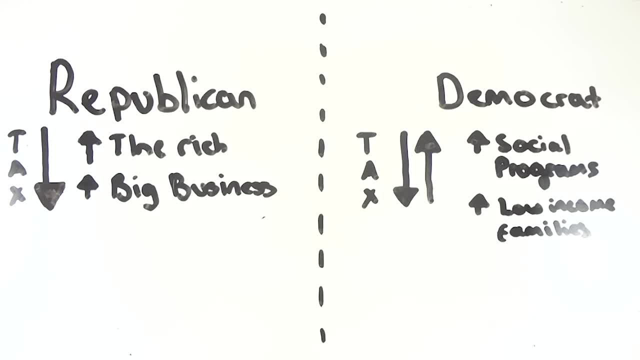 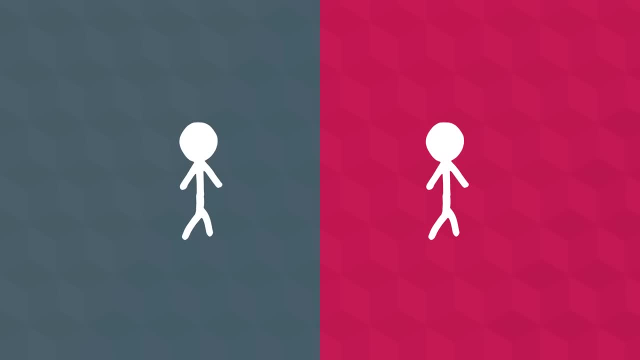 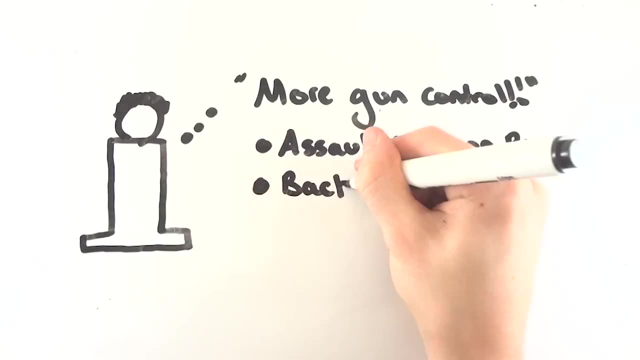 wealthy and big businesses, whereas the Democrats support progressive taxes to help fund social programs and to help out lower income citizens. Gun laws, An issue which divides many Americans, also divides Republicans and Democrats. Democrats favour more gun control, but recognise that the American amendment is an important part of American tradition and that the right 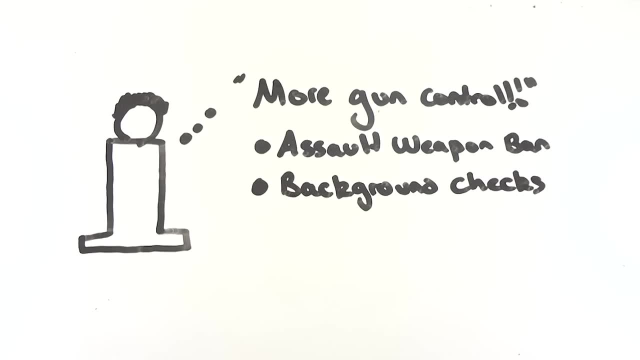 to own and use firearms should be preserved. Reinstating the assault weapon ban and working to make the background check system stronger so that guns aren't getting into the hands of the irresponsible are high up the agenda for the Democrats. The Republicans, on the other hand, oppose gun control laws and go as far to say that they believe you should. 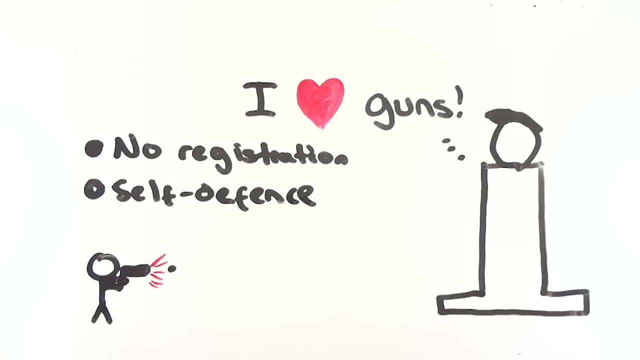 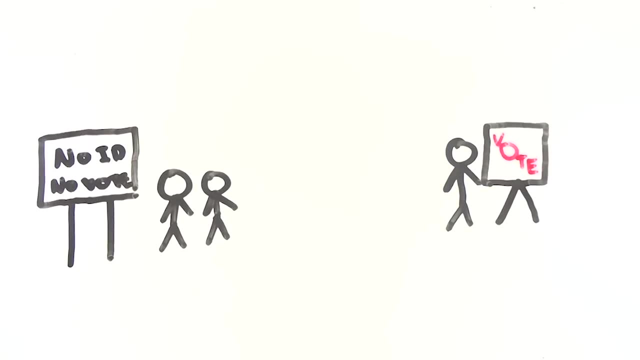 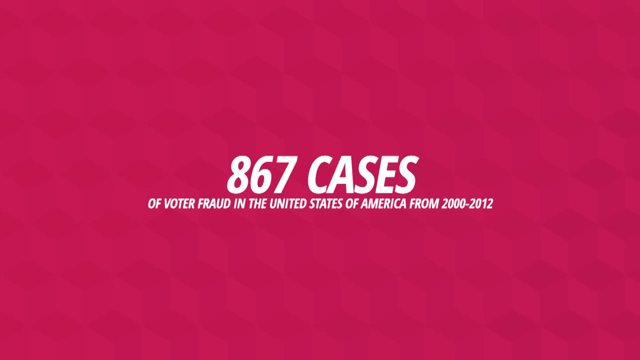 be able to obtain and store ammunition without registration, and they support the right to self-defence Voter ID laws. The Republican party is currently pushing for elections to require a photo identification for voting to, in their words, prevent election fraud. Between 2000 and 2012, there were 867 cases of voter fraud, but the Republicans 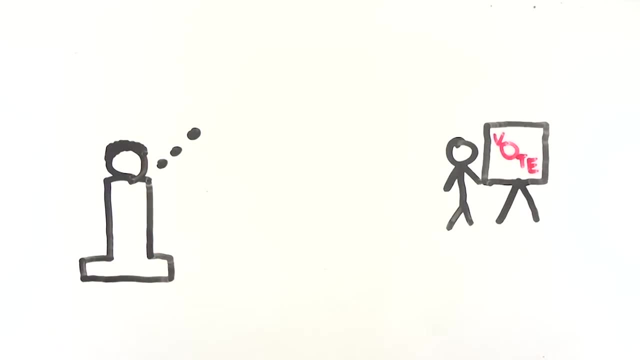 want this to be zero. The Democrat party are complete opposites on voter identification laws, saying that they believe everyone has the right to vote, making them in opposition of laws which begin to put restrictions on those trying to vote. According to the Democrats, 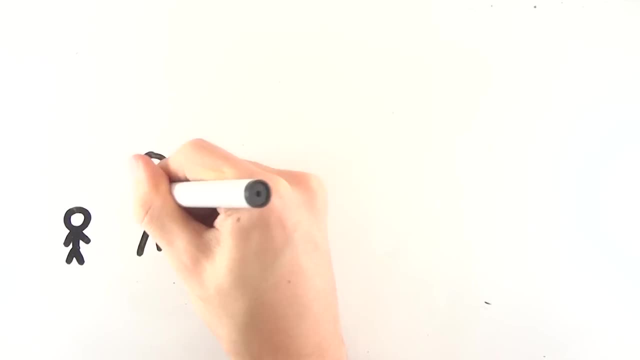 introducing photo identification would affect young voters, people of colour, lowering the income, low income families, those with disabilities and the elderly, which is a large number of voters who wouldn't be able to vote and have their opinion hurt. Pro-life versus choice, As I'm sure you can begin to tell the Republican. 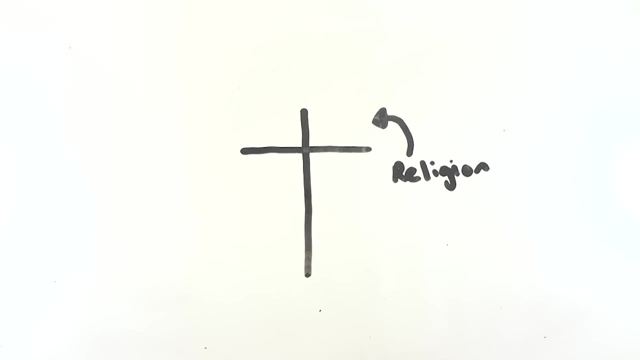 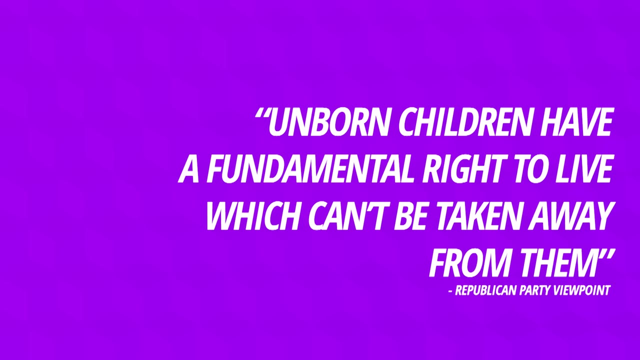 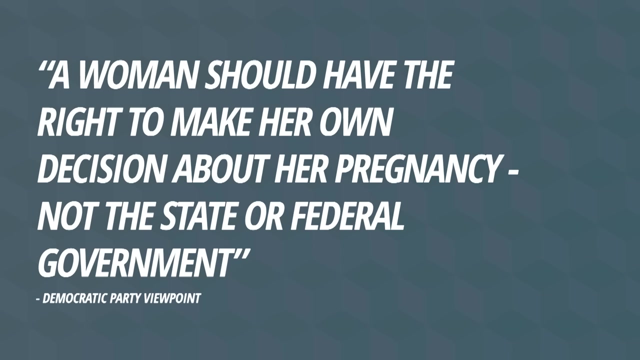 party is very much influenced through religion and tradition, which would make it no surprise that they support the government restricting abortions. The Republicans believe that unborn children should have the fundamental right to live, which cannot be taken away from them. The Democrats, on the other hand, support Roe versus Wade and believe that a woman should 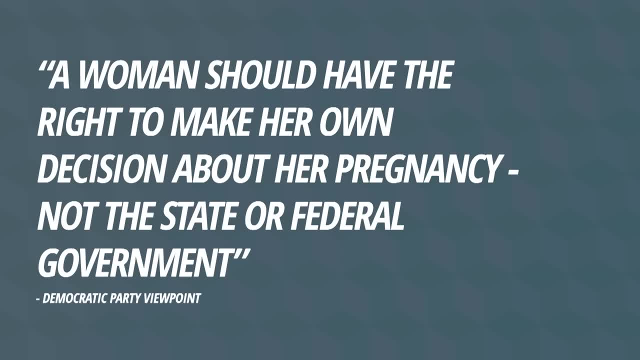 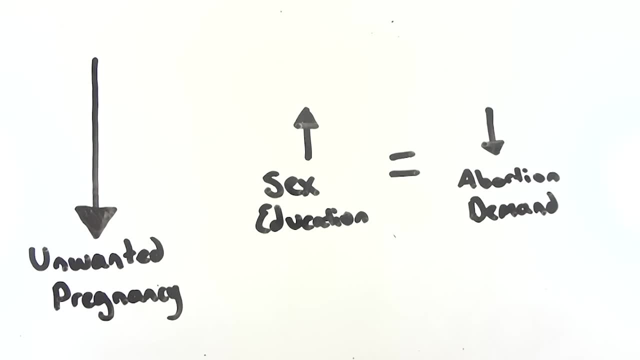 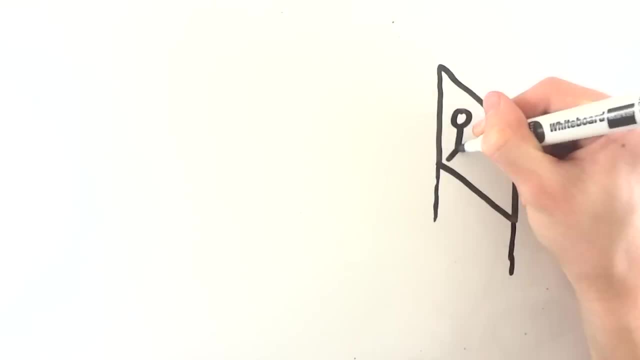 have the right to make her own decisions about her pregnancy and that politicians and the government have no right to get involved with a woman's pregnancy. The Democrat party also wants to help reduce the number of unwanted pregnancies through better sex education, which should then help decrease the need for abortions. STD rates are hitting all time highs in the 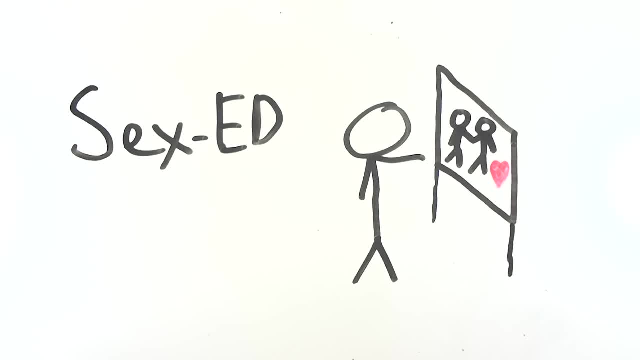 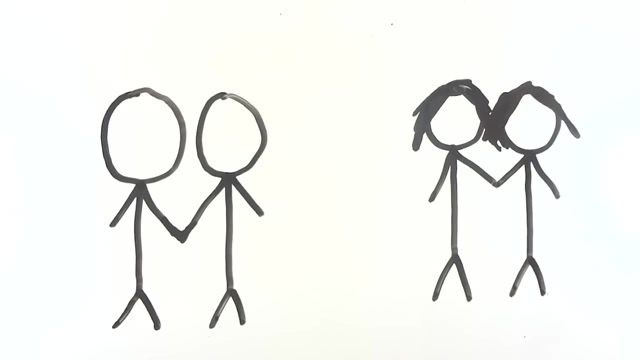 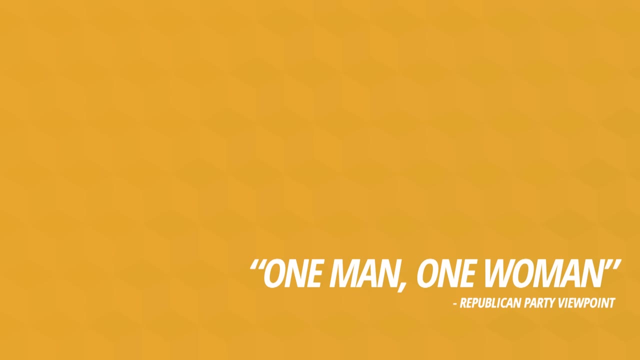 USA, so putting work into sex education is something which the Democrats believe will benefit society greatly. Same sex marriages Being very traditional and religious based, it's a very common practice to not recognise same sex relationships. with the party aiming to constitutionally define marriage as one man and one woman, The Republicans also have 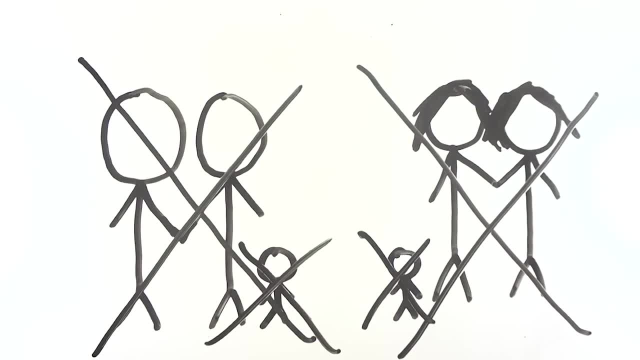 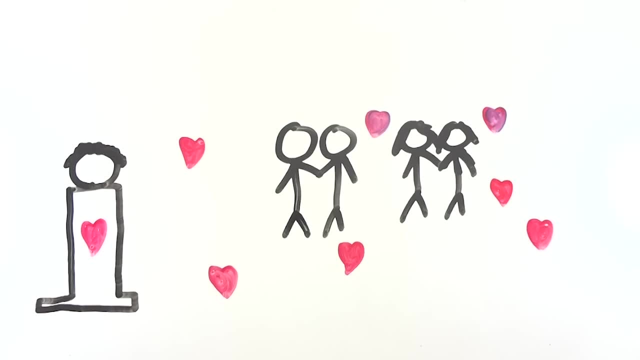 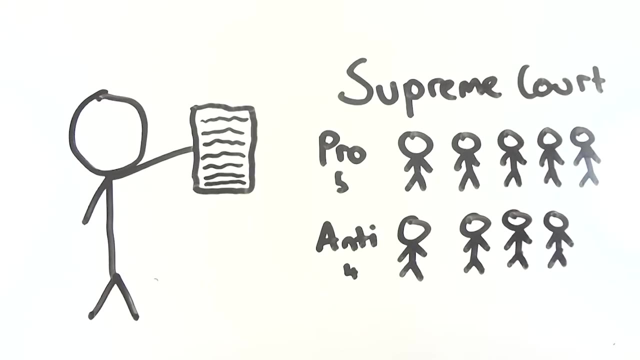 the viewpoint that same sex couples should not be able to adopt children. The Democrats oppose same sex discrimination on the federal and state level and believe that same sex couples should receive the same amount of respect and legal treatment as heterosexual couples. In fact, it was under the Democratic Obama administration that Section 3 of the 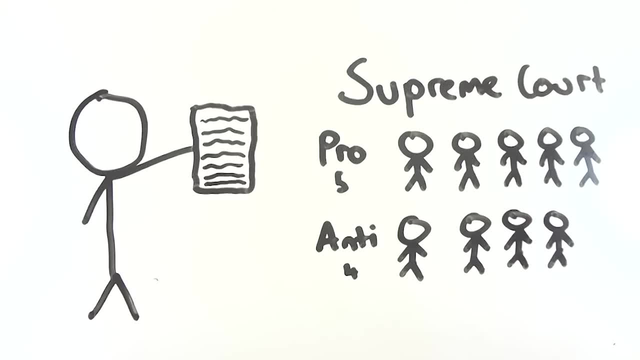 Defence of Marriage Act, which defined marriage as a union of two sexes, was passed. This decision between a man and a woman was found to be unconstitutional, a decision which was ruled by the Supreme Court on June 26, 2013.. Limit of Government Republicans have positioned themselves into. 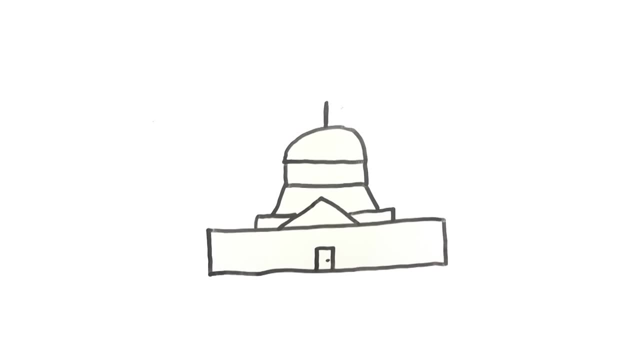 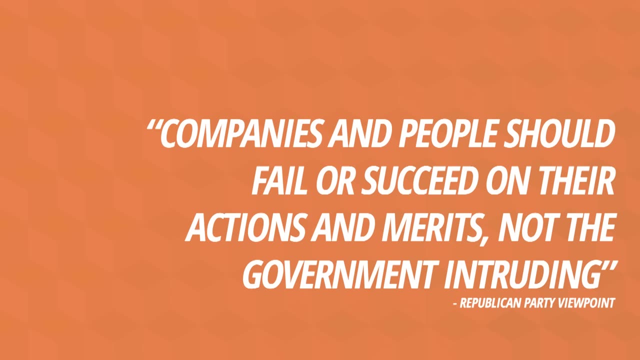 believing that a smaller government is better, with Republicans preferring themselves to have less responsibilities in society, and that they should let people and companies fail or succeed based on their merits and actions, instead of the government intruding. The Republican party don't like policies which essentially allow the government to have the power to pick and choose the winners and losers. The Republican party don't like policies which essentially allow the government to have the power to pick and choose the winners and losers. Therefore harmonization of them or the losses of the market, instead letting economies 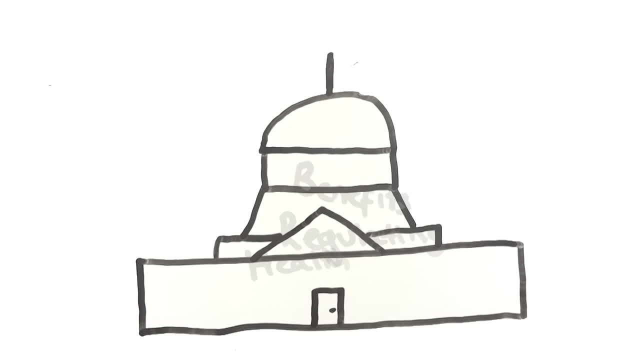 and businesses speak for themselves has become in WA. The Democrats, on the other hand, believe that the Federal Government should have a stronger role in helping Americans with the challenges they face, whether it be through regulating businesses, being more involved with healthcare benefits or other programs.